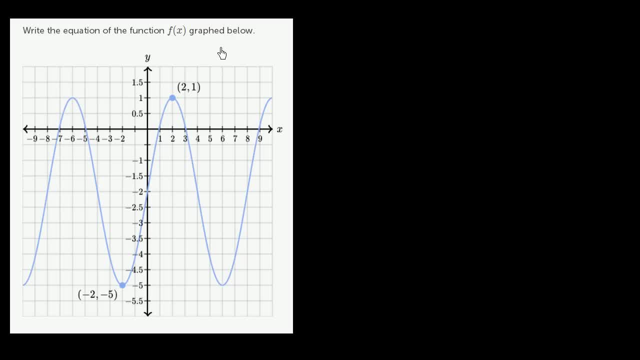 Write the equation of the function f of x graphed below. So we have this clearly periodic function. So immediately you might say: well, this is either going to be a sine function or a cosine function. But its midline and its amplitude are not just the plain vanilla sine or cosine function. 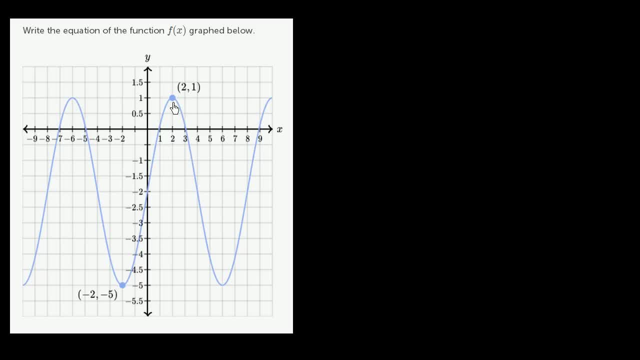 And we can see that right over here The midline is halfway between the maximum point and the minimum point. The maximum point right over here it hits a value of y equals 1.. At the minimum point it hits a value of y is equal to negative 5.. 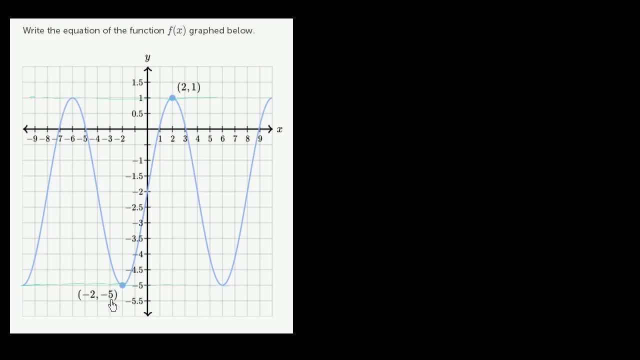 So halfway between those, the average of 1 and negative 5, 1 plus negative 5 is negative. 4 divided by 2, is negative 2.. So this right over here is the midline. So this thing is clearly. so this is: y is equal to negative 2.. 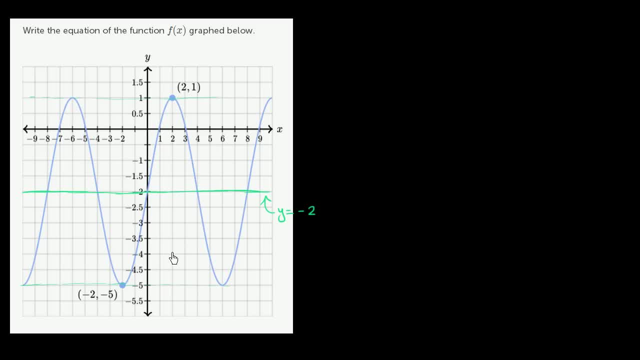 This is y is equal to negative 2. So it's clearly shifted down. So actually I'll talk in a second about what type of an expression it might be, But now also let's think about its amplitude. Its amplitude, that's how far it might get away. 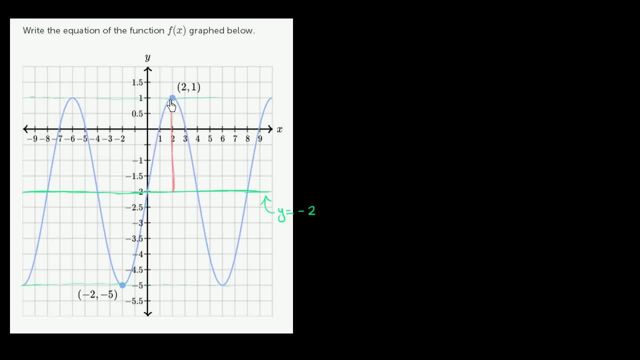 from the midline We see here. it went 3 above the midline, going from negative 2 to 1.. It went 3 above the midline at the maximum point And it can also go 3 below the midline at the minimum point. 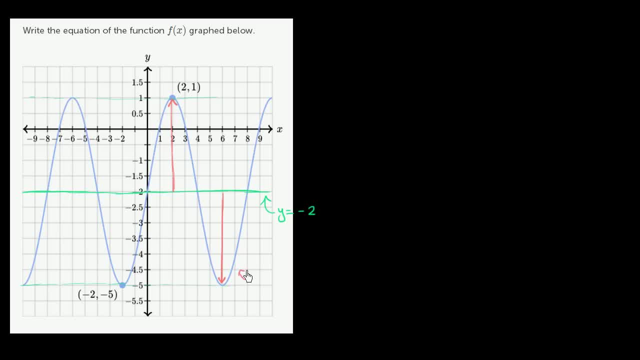 So this thing clearly has an amplitude of 3.. So amplitude of 3.. So immediately we can say: well, look, this is going to have a form, something like f of x. So f of x is equal to the amplitude 3.. 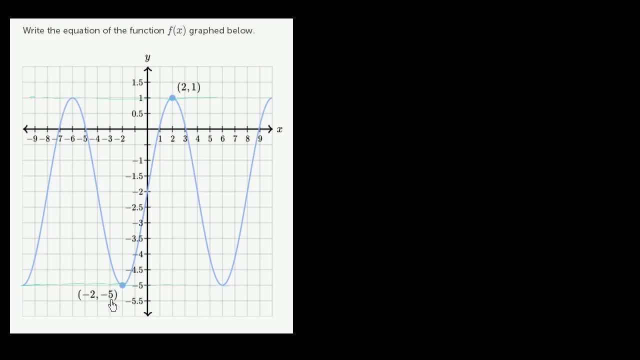 So halfway between those, the average of 1 and negative 5, 1 plus negative 5 is negative. 4 divided by 2, is negative 2.. So this right over here is the midline. So this thing is clearly. so this is: y is equal to negative 2.. 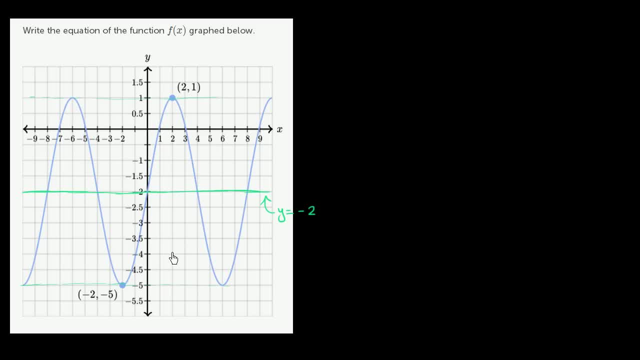 This is y is equal to negative 2. So it's clearly shifted down. So actually I'll talk in a second about what type of an expression it might be, But now also let's think about its amplitude. Its amplitude, that's how far it might get away. 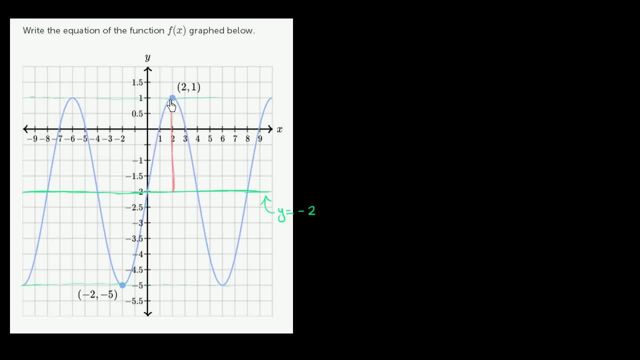 from the midline We see here. it went 3 above the midline, going from negative 2 to 1.. It went 3 above the midline at the maximum point And it can also go 3 below the midline at the minimum point. 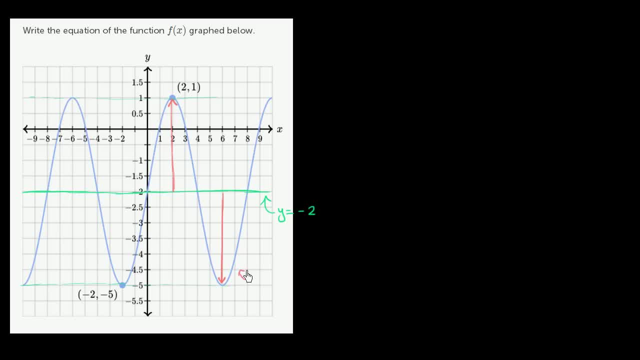 So this thing clearly has an amplitude of 3.. So amplitude of 3.. So immediately we can say: well, look, this is going to have a form, something like f of x. So f of x is equal to the amplitude 3.. 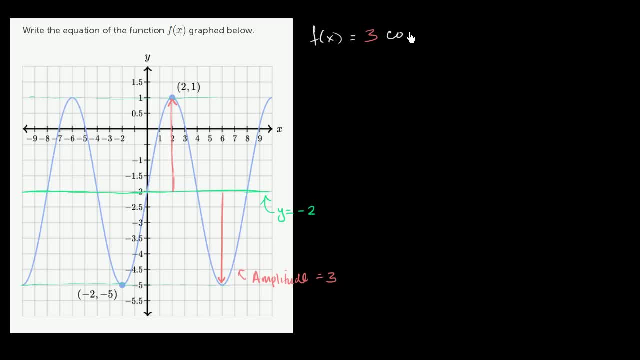 We haven't figured out yet whether this is going to be a cosine function or a sine function, So I'll write cosine first. Cosine may be some coefficient times x plus the midline. The midline we already figured out was minus 2 or negative 2.. 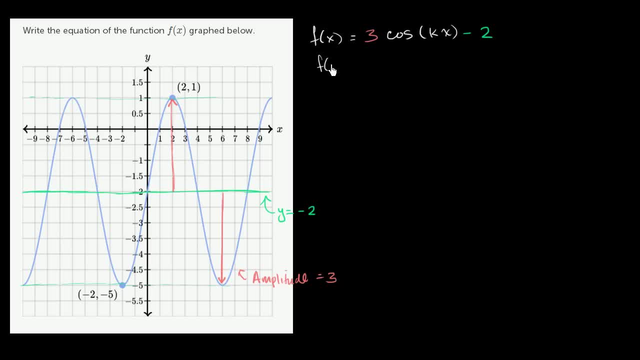 So it could take that form. Or it could take: f of x is equal to 3 times, It could be sine of x, It could be sine of x, It could be sine of x Or sine of some coefficient times: x Sine of kx minus 2 plus the midline, so minus 2.. 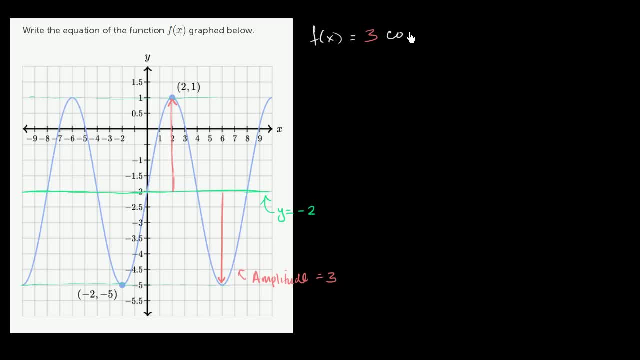 We haven't figured out yet whether this is going to be a cosine function or a sine function, So I'll write cosine first. Cosine may be some coefficient times x plus the midline. The midline we already figured out was minus 2 or negative 2.. 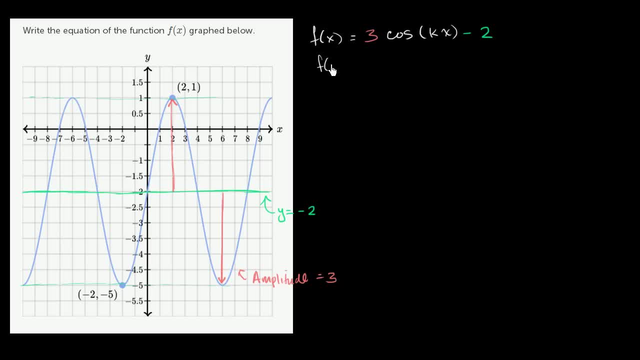 So it could take that form. Or it could take: f of x is equal to 3 times, It could be sine of x, It could be sine of x, It could be sine of x Or sine of some coefficient times: x Sine of kx minus 2 plus the midline, so minus 2.. 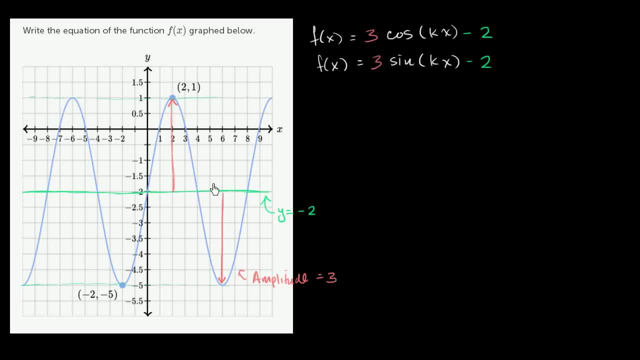 So how do we figure out which of these are? Well, let's just think about the behavior of this function when x is equal to 0.. When x is equal to 0, if this is kx- then the input into the cosine is going to be 0. 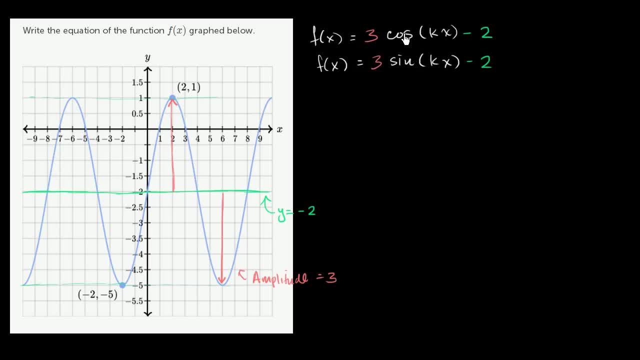 Cosine of 0 is 1,. whether you're talking about degrees or radians, cosine of 0 is 1.. While sine of 0, so if x is 0, k times 0 is going to be 0.. Sine of 0 is 0.. 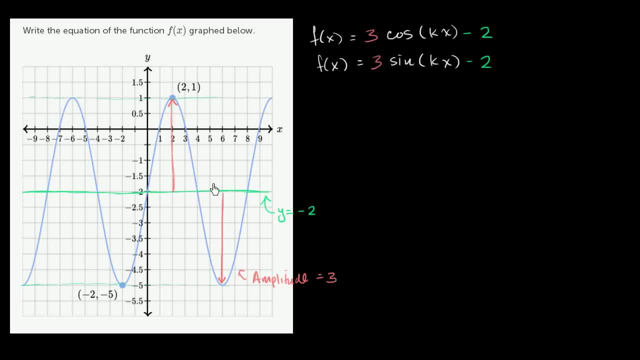 So how do we figure out which of these are? Well, let's just think about the behavior of this function when x is equal to 0.. When x is equal to 0, if this is kx- then the input into the cosine is going to be 0. 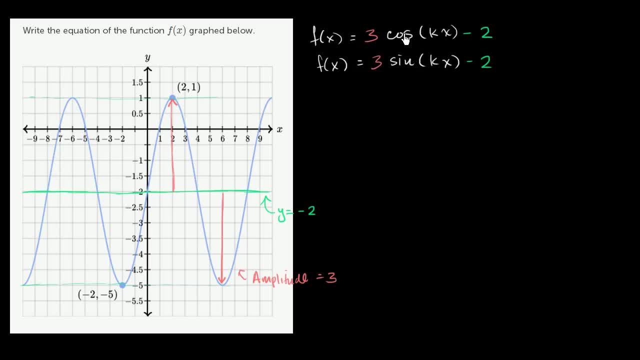 Cosine of 0 is 1,. whether you're talking about degrees or radians, cosine of 0 is 1.. While sine of 0, so if x is 0, k times 0 is going to be 0.. Sine of 0 is 0.. 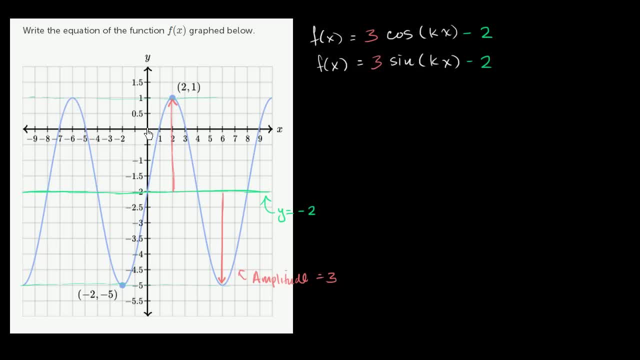 So what's this thing doing when x is equal to 0?? Well, when x is equal to 0, we are at the midline. If we're at the midline, that means that all of this stuff right over here evaluated to 0.. 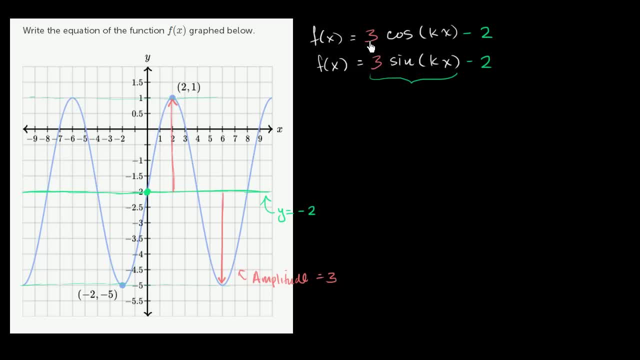 So since when x equals 0, all of this stuff evaluated to 0, we can rule out the cosine function When x equals 0, here this stuff doesn't evaluate to 0. So we can rule out this one right over there. 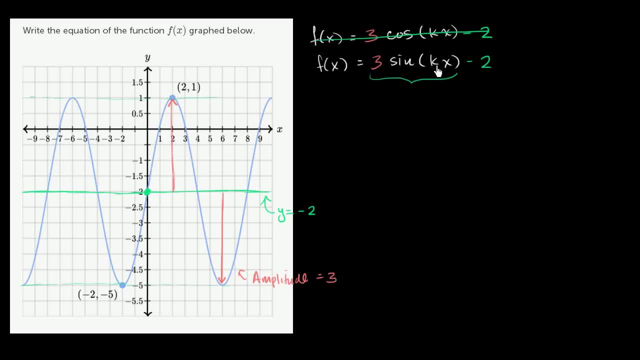 And so we are left with this And we just really need to figure out: what is this? What could this constant actually be? And to think about that, let's look at the period of this function. So to go from, and we could, let's see. 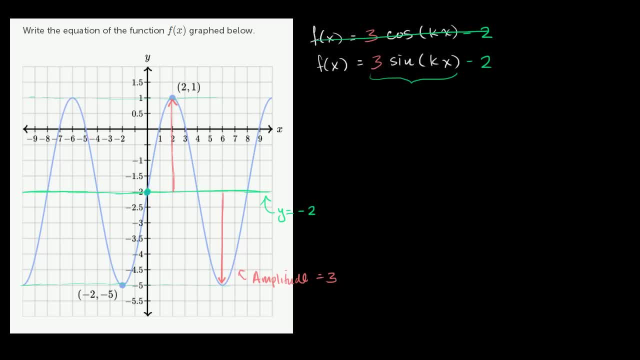 if we went from this point where we intersect the midline. we go this point to intersect the midline and we have a positive slope. the next point that we do that is right over here. So our period is 8.. So what coefficient could we have here? 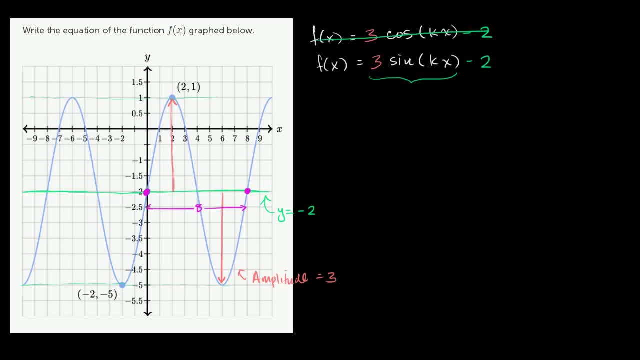 to make the period of this thing be equal to 8?? Well, let's just remind ourselves what the period of sine of x is. So the period of sine of x- so I'll write period right over here- is 2 pi. 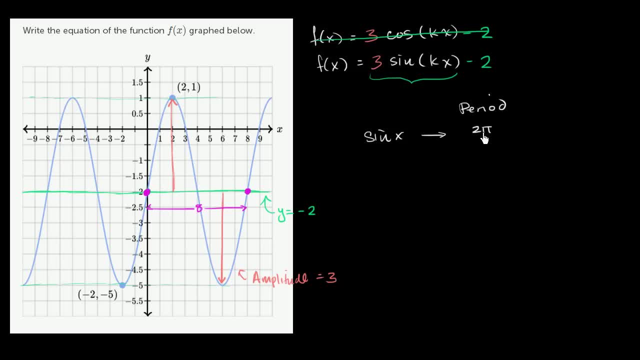 2 pi. you increase your angle by 2 pi radians or decrease it. You're back at the same point on the unit circle. So what would be the period of sine of kx? Well, now, your x, your input, which? 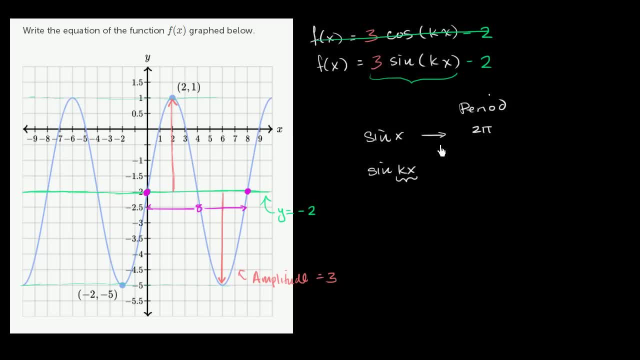 is increasing k times faster, So you're going to get to the same point k times faster, so your period is going to be one kth as long. So now your period is going to be 2 pi over k. Notice you're increasing your argument as x increases. 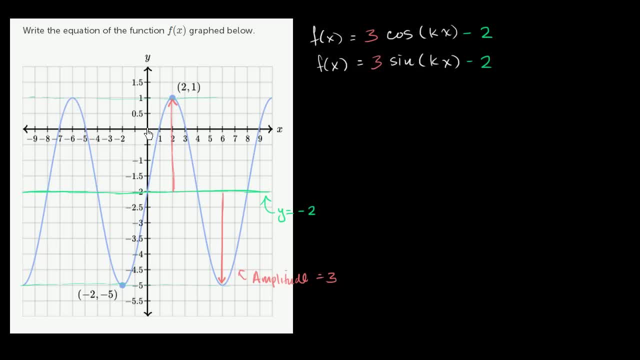 So what's this thing doing when x is equal to 0?? Well, when x is equal to 0, we are at the midline. If we're at the midline, that means that all of this stuff right over here evaluated to 0.. 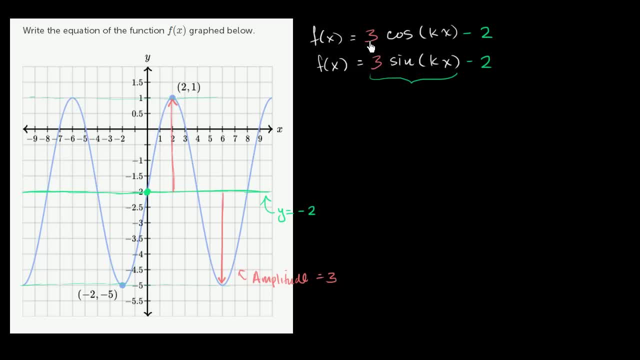 So since when x equals 0, all of this stuff evaluated to 0, we can rule out the cosine function When x equals 0, here this stuff doesn't evaluate to 0. So we can rule out this one right over there. 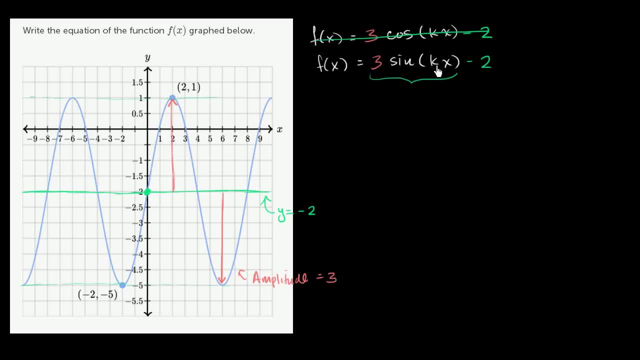 And so we are left with this And we just really need to figure out: what is this? What could this constant actually be? And to think about that, let's look at the period of this function. So to go from, and we could, let's see. 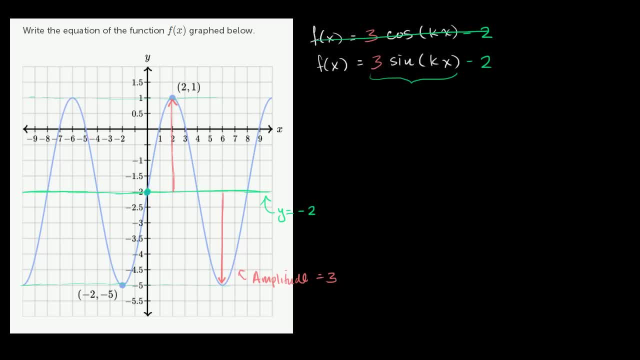 if we went from this point where we intersect the midline. we go this point to intersect the midline and we have a positive slope. the next point that we do that is right over here. So our period is 8.. So what coefficient could we have here? 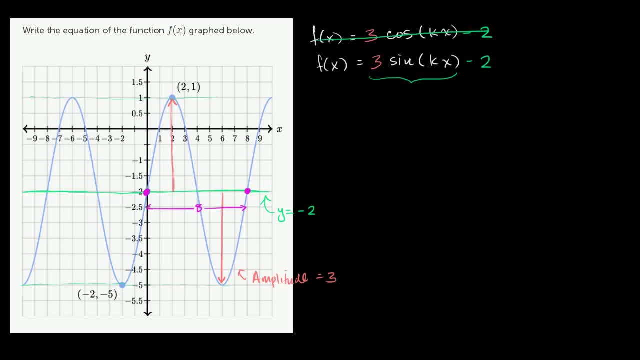 to make the period of this thing be equal to 8?? Well, let's just remind ourselves what the period of sine of x is. So the period of sine of x- so I'll write period right over here- is 2 pi. 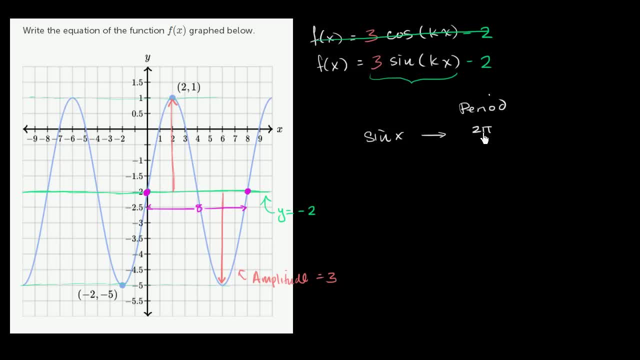 2 pi. you increase your angle by 2 pi radians or decrease it. You're back at the same point on the unit circle. So what would be the period of sine of kx? Well, now your x, your input, is increasing k times faster. 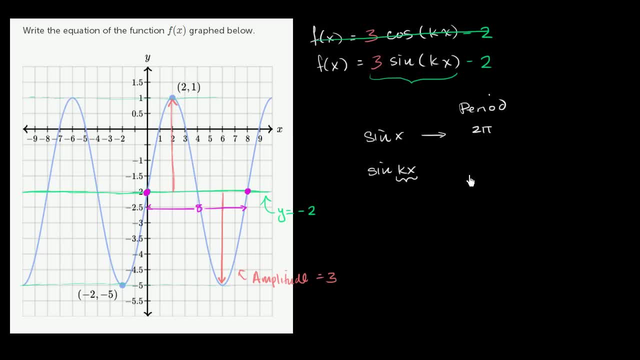 So you're going to get to the same point k times faster. So your period is going to be 1 kth as long. So now your period is going to be 2 pi over k. Notice you're increasing your argument as x increases your argument into the sine function. 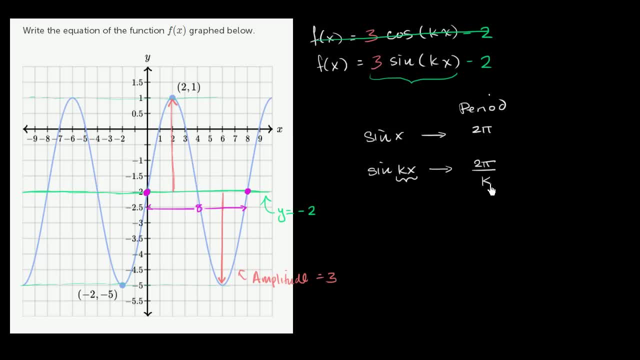 is increasing k times as fast. You're multiplying it by k, So your period is going to be shorter. it's going to take you less distance to get for the whole argument Right. So your period is going to be 2 pi over k. 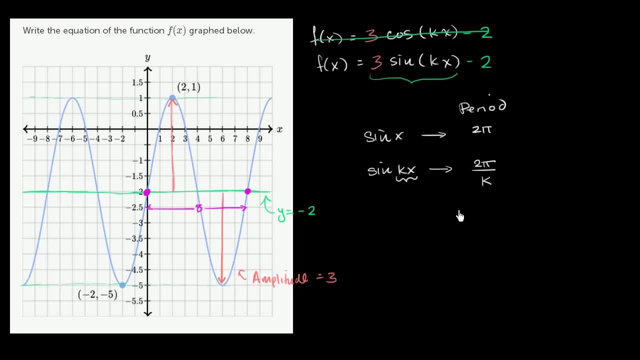 Okay, to get to the same point on the unit circle. So let's think about it this way Now. so if we wanted to say two pi over k is equal to eight, so if two pi over k is equal to eight, well, what is our k? 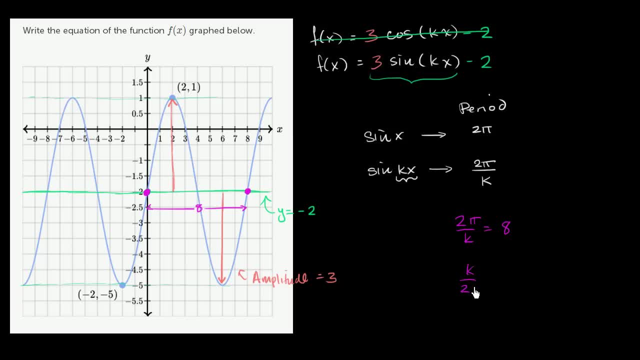 Well, we could take the reciprocal of both sides. We get k over two pi is equal to one over eight. Multiply both sides by two pi and we get k is equal to. let's see, this is one, this is four. 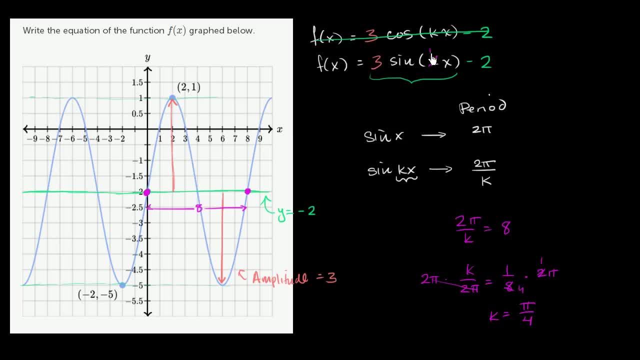 k is equal to pi over four. And we are done- and you can verify that by trying out some of these points right over here- that this function is equal to three sine of pi over four x minus two. 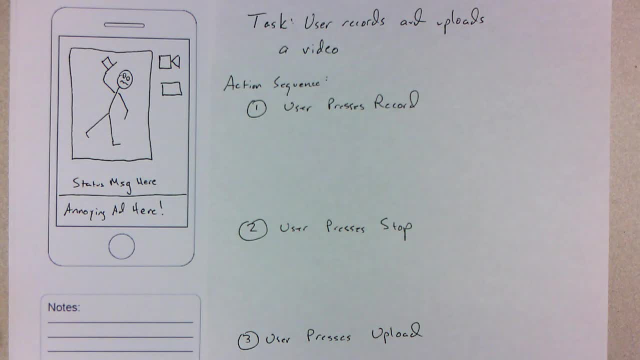 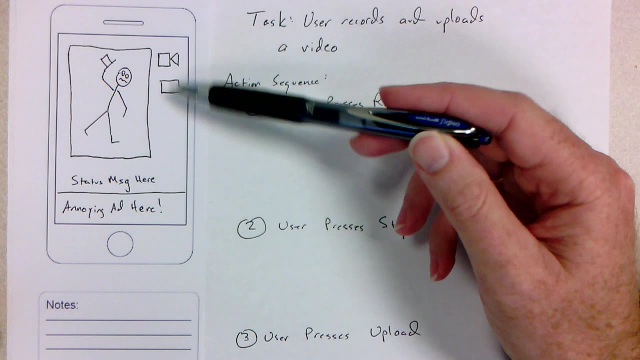 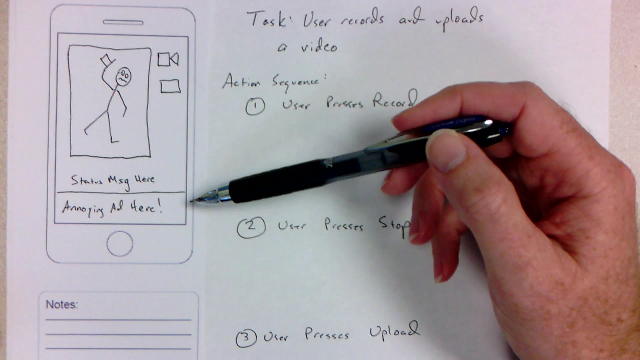 Okay, this is a sample of a cognitive walkthrough. What I have is a paper prototype for a single screen application. It's an iPhone app, so there's a nifty prototype here on this nifty iPhone screen printout I have. There's a link to this kind of stuff on our Canvas site. 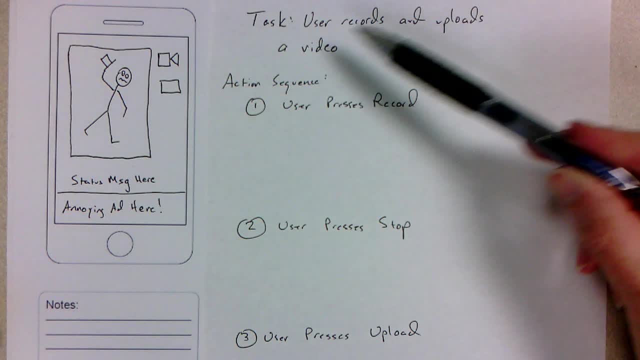 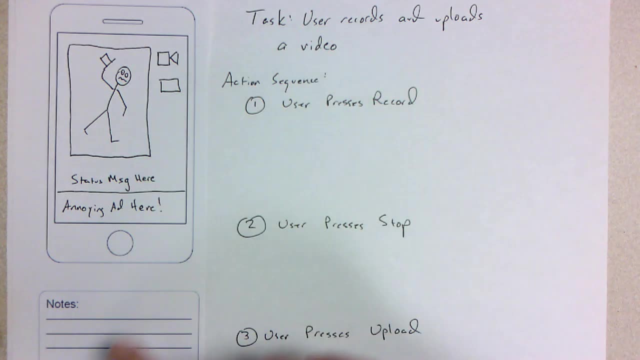 All this is this: records a video. Like we can see here, the task is for a user to record and then upload a video. So basically, they press record boop, they record, press stop boop and then they're going to upload. 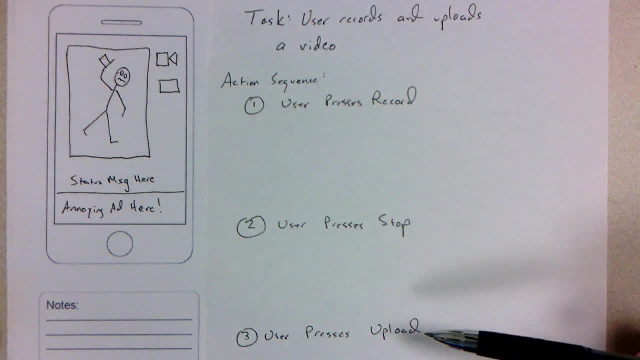 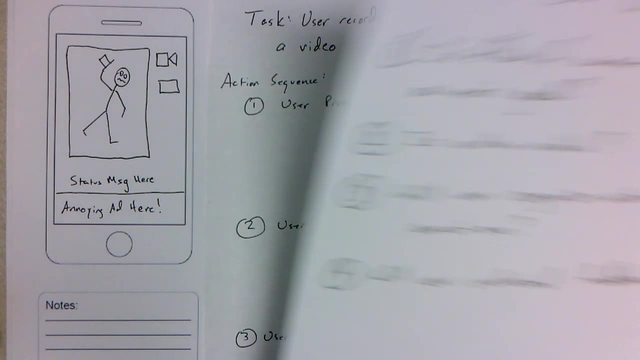 So we have an action sequence of three steps for the cognitive walkthrough. We need to write down the action sequence first, and then for every one of those actions we're going to ask four questions. So the four questions we ask, these are kind of written in plain English. 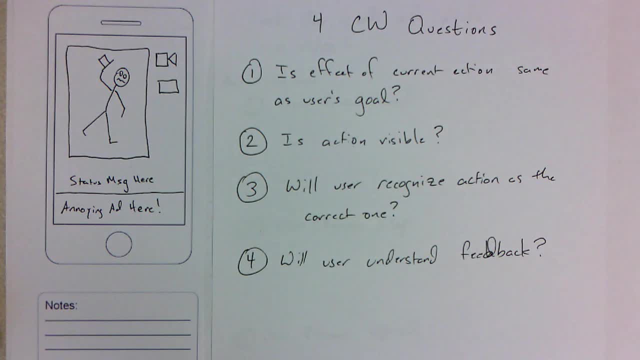 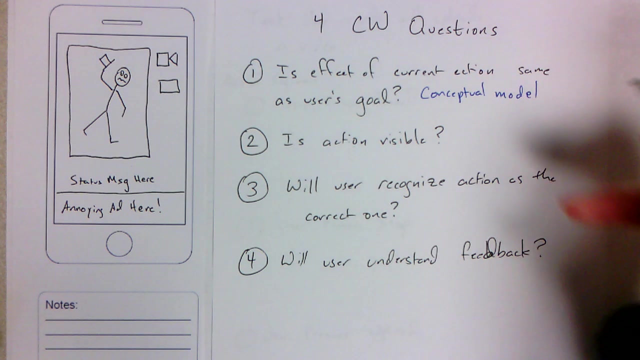 Instead of the slightly more confusing version that our reading had, And so what they have to do for the action we're looking at right then is the user on the right track. So do they have the right conceptual model? so they're trying to do the right thing at the right time. So that's basically what the first one's getting at. 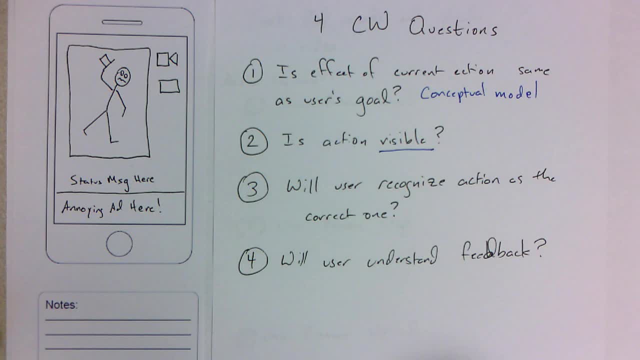 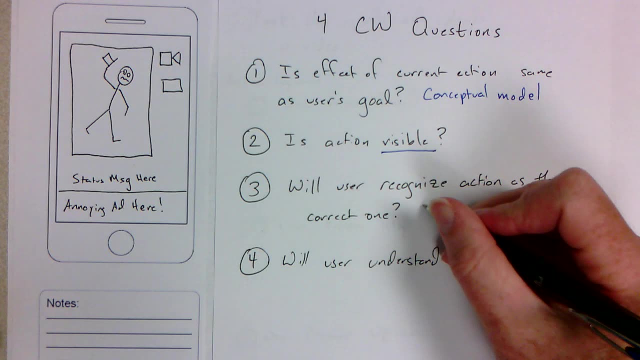 The second one. just once they know what they're doing, can they see what they need to do? Is it there on the screen for them to access? Then the third question has to do with labeling. So will the user recognize even though it's on the screen? will they recognize it's the right one.